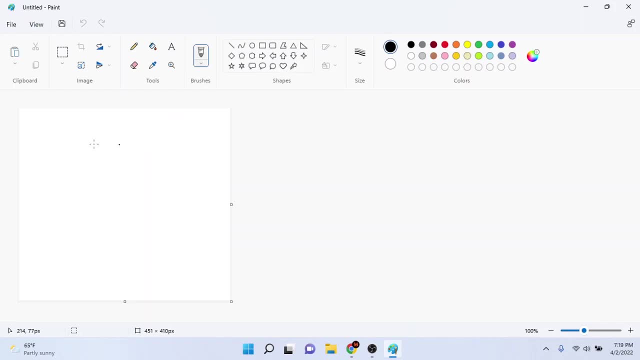 let's say we have um, let's go on paint. let's say we have some intervals. so what I mean by interval? I mean it could be like a time that with a start and end, it could be, I don't know, a line segment with a start and end. so essentially, anything that's like like has like a start and an end. 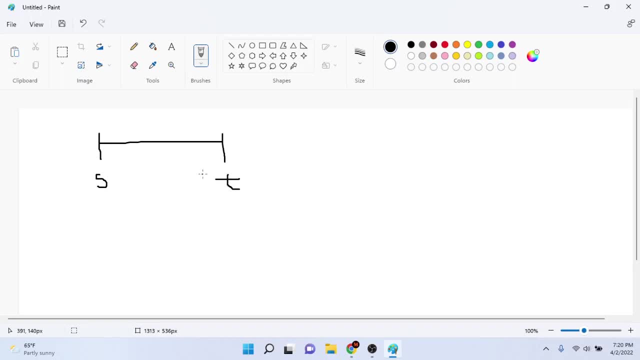 right, it could be a time. it could be like like a start time and end time, like anything like this. right, it could be on a number line. so let's say I had like an interval between one and five, right? so let's say we want to check and, uh, let's say I have another interval, let's say between two and. 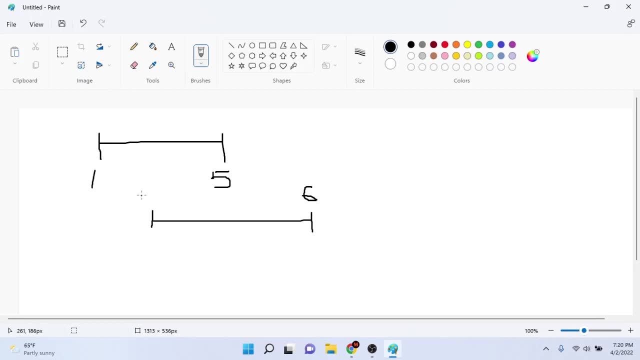 six, right, so two and six. so this would be two and six and this would be one and five. now, um, in like some books to check if something's overlapping right. so how would you do it if you wanted to check if something's overlapping right? well, um, what some people would do is they would check. 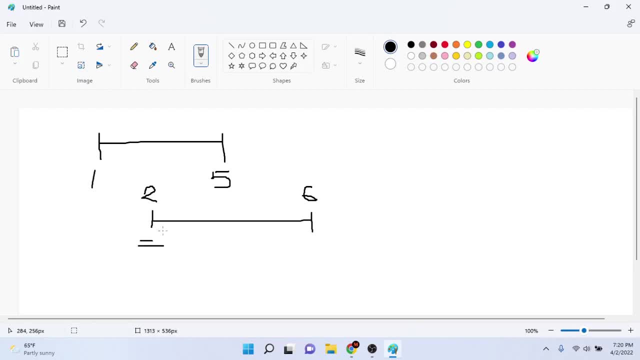 like the, the left most, the most boundaries, to see if it's between the starting boundary for one of them, if it's greater than the left side of one of the starting boundaries and smaller than the right side of the starting boundaries, right, and then you could do. 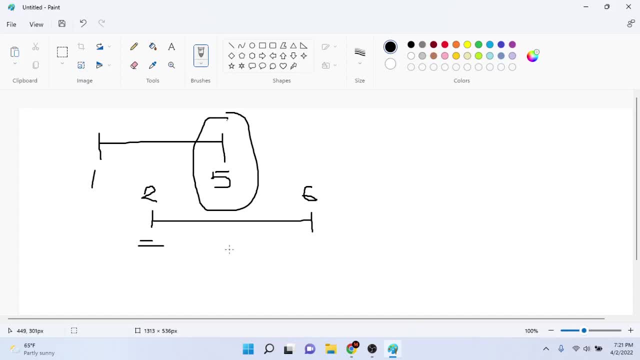 that that is a. that is a way to do it to check for boundaries, and I know I know some people they also check. if, like, the right side of this boundary is between these two boundaries, right, then that means they're overlapping right there between the start and end time. right, these two intervals are between, but 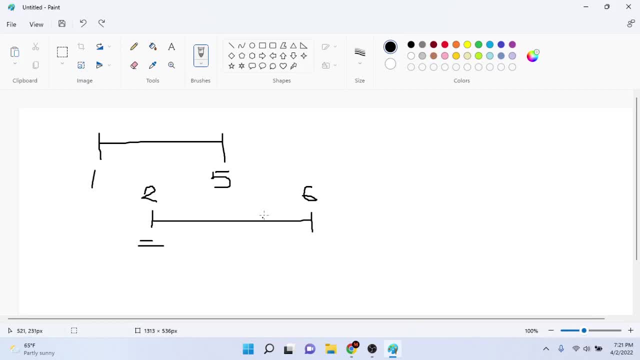 here's a trick that you could do that I learned in this add coder problem is that all you have to do is just check if the maximum between the left boundaries, so the maximum of these maximum of this boundary, is smaller than or equal to the minimum of this boundary of the right boundary. so in this case it would be the 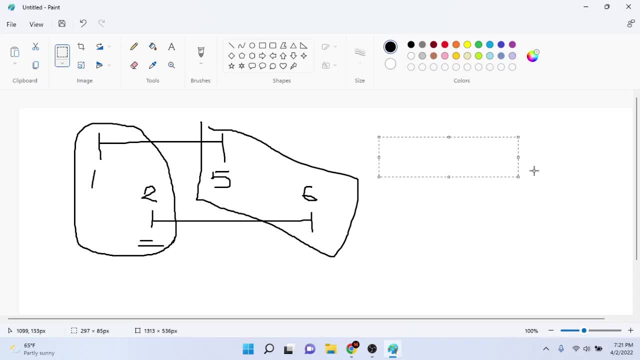 maximum of the left boundary and the maximum of the right boundary and the minimum of the right boundary and the maximum of the right boundary and the- I'll just type it out here: it would be the max- whoops, it'd be the max between the left boundaries, which would be 1 & 2- is a less than or equal to the minimum of the. 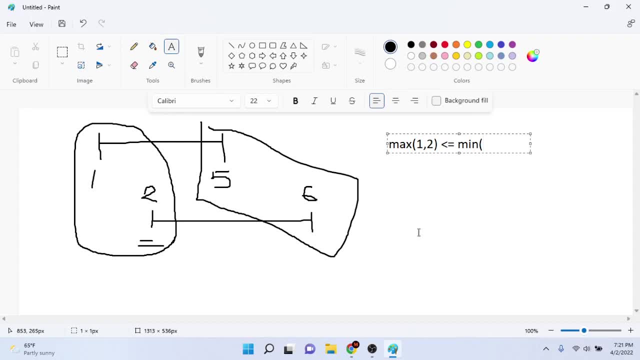 right boundary, which would be 5 & 6. okay, and the reason why this works is because if the maximum of 1 & 2, which would be 2 in this case, this would be 2 here, if it's smaller than or equal to the minimum of the right boundary is. 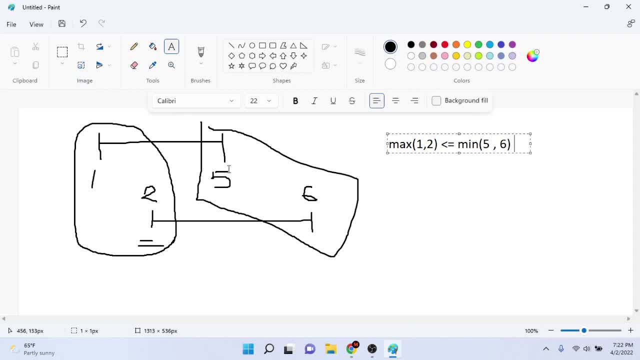 The right boundary of the right boundaries of 5 and 6 is 5.. So since 2 is less than or equal to 5, that's overlapping And this works in most cases. actually, If you had another interval, let's say we had here, let's say we had 1 and 5.. 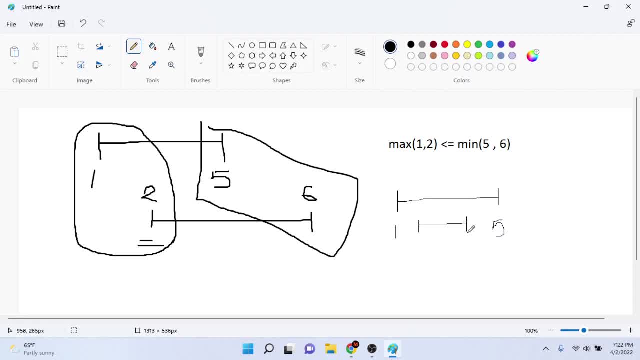 And then we have another interval like 2 to 3, right? So this interval is overlapping, right? So if I were to check the max between the left boundaries, which is 1 and 2, so this max of 1 and 2, it would be 2, right. 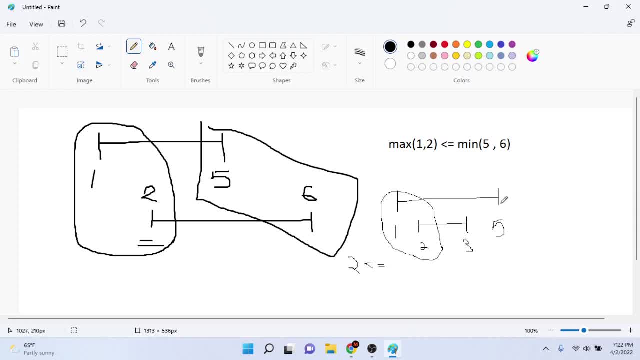 And 2 is smaller than or equal to the minimum of 2 and 5, that's between 3 and 5 of the right boundaries, right? So then that would be 3,, right? The minimum between 3 and 5 is 3.. 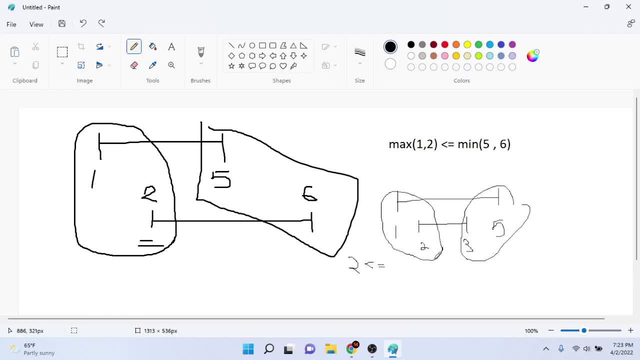 And that's also overlapping right. So that would be an overlapping interval also. So yeah, as long as So. if you check the maximum of the left boundaries less than or equal to the minimum of the right boundaries, this trick works regardless, okay. 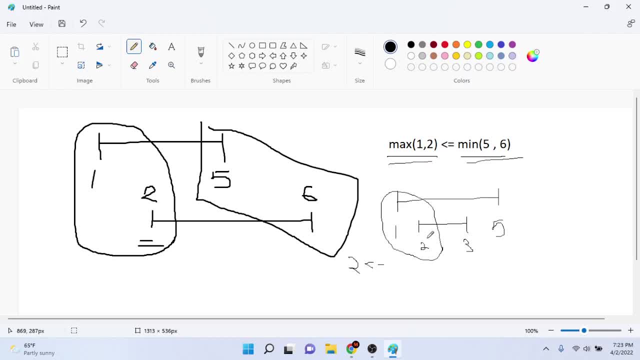 You don't have to do any of these conditionals of if the left boundary is greater than or equal to the left side of one interval and smaller than or equal to the right side, and if the right boundary is greater than or equal to the left boundaries. 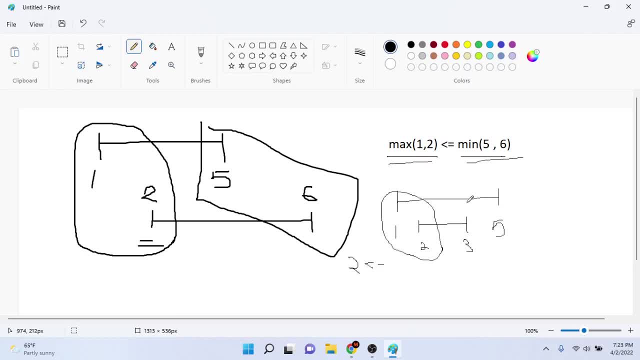 and smaller than or equal to the right one. right The second one, you don't have to check if I don't know. the left boundary is equal to the left boundary and the right boundary is smaller than or equal to the right boundary. 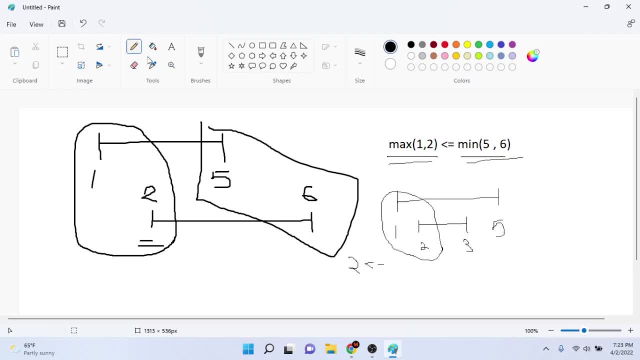 Like you don't need to do all this interval checking. Yeah, so all you have to do is, if I were to write this, rewrite this again. there's a cool trick. you just have to do min max of left boundary bound.